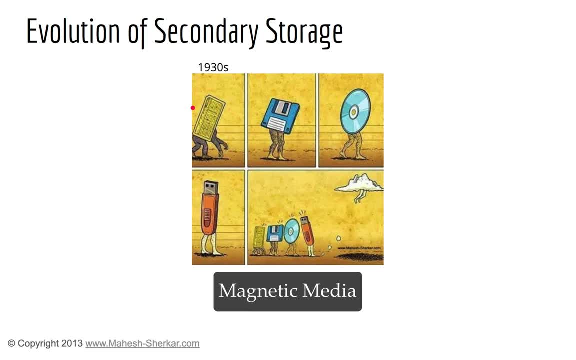 60s, again not shown in this picture, but in a different format: Hard disk drives, which is so much faster than tape drives because a hard drive continues to spin at higher speed. Then, in the 70s and 80s, floppy drives of various sizes were used, starting with 8-inch. 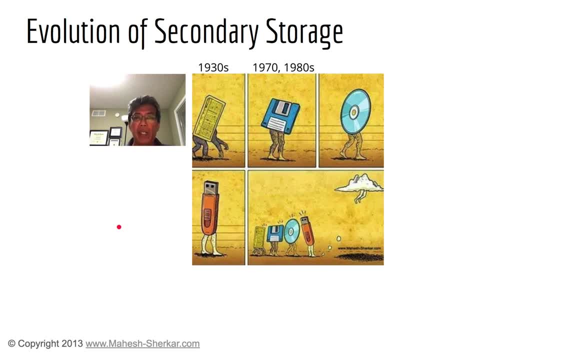 drive, then a 5 ¼-inch drive and then later to a 3.5-inch drive In the 60s, again not shown in this picture but in a different format. hard disk drives 90s- non-magnetic storage mediums- were becoming popular during the time like. 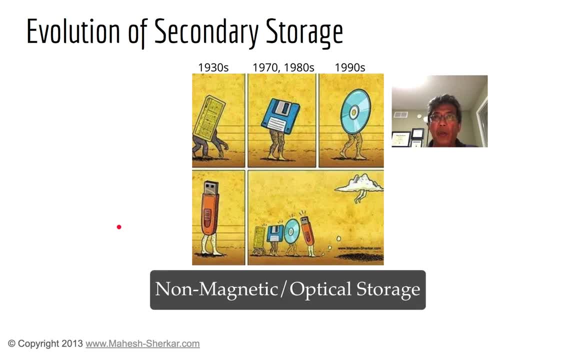 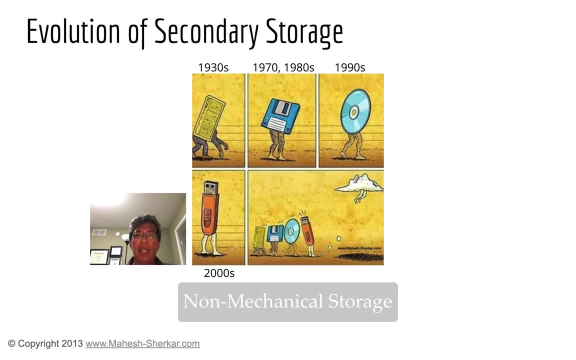 CD-ROMs- writable CDs and DVDs- were widely used for distributing software and also for backups, And in the 2000s the trend was to use non-mechanical storage devices because they are more reliable and also faster. And finally, we see how cloud storage is the norm today. In the previous module, when we talked 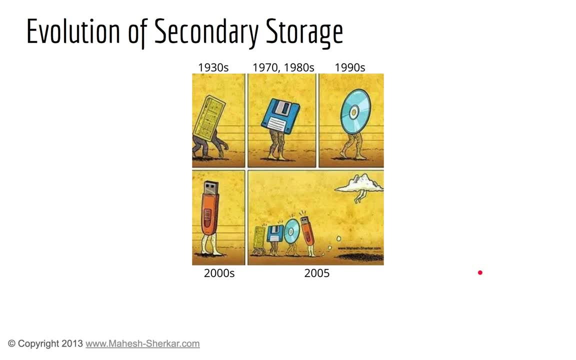 about file system interface. we don't really care whether the data is from a floppy-drive, a CD-ROM, DVD or a remote storage. In this module, when we talk about file system implementation, we will see the chain of operations when a program attempts to access a file. 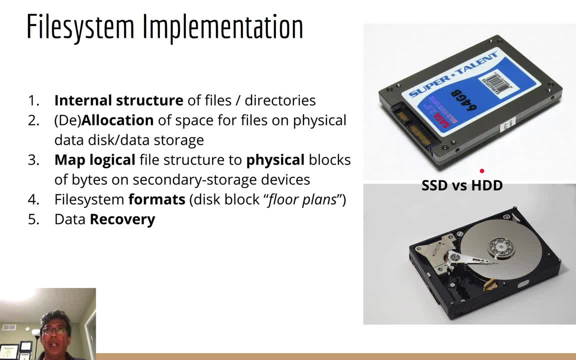 There are five major types of file system topics related to file system implementation. first we're going to look at the internal structure of files and directories and then next we're going to look at different technique to allocate or deallocate space needed for files on physical disk or storage, and also we will see how 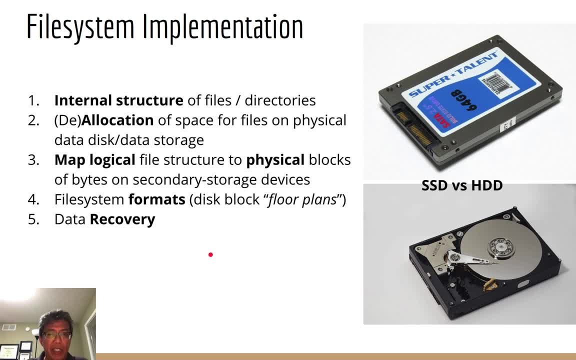 the file system will perform mapping from logical file structures to physical blocks of bytes on the storage, and we also look at what is the meaning of file system format. so let's say we're gonna see how V fat is different from the exit to or from NTFS. and then the last topic, important topic. 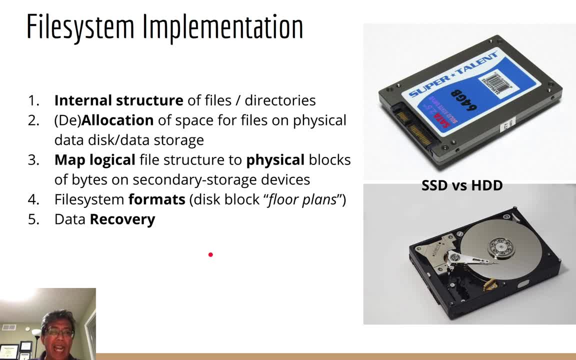 is how we recover corrupted data, because at times, operations to your storage device may not be able to complete and that will create an inconsistent state of your data. and just to remind you, when we talk about a storage device, we can either refer to a solid state drive or a hard disk drive. from our discussion about processor management and 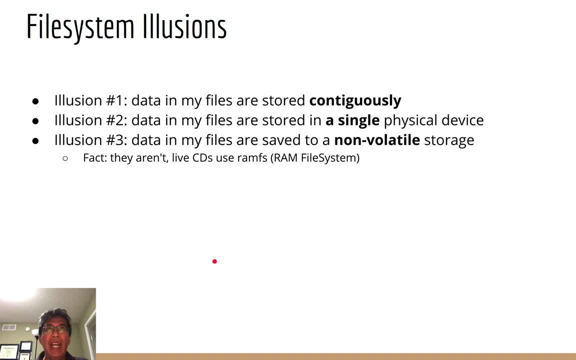 memory management. we see a few examples how our operating system creates many different illusions, and then the goal is to present a programming model that is easy for the user to use. we'll continue to see more illusions. when the operating system handles file operations, for instance, the first illusion, the user will think that their data are always. 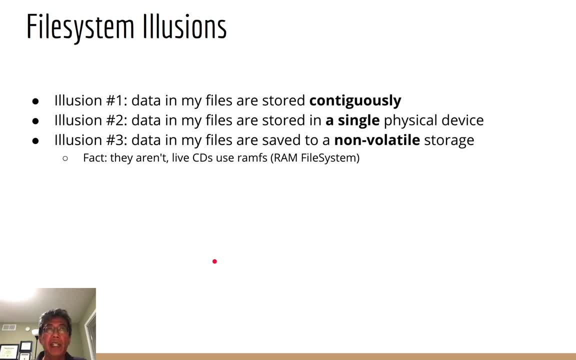 contiguous. and then the second: their data may be stored into a single physical device. and then third illusion is that they will think that their data are always saved to a non-volatile storage, but in fact this is not true because, for instance, when you try to install a new operating, 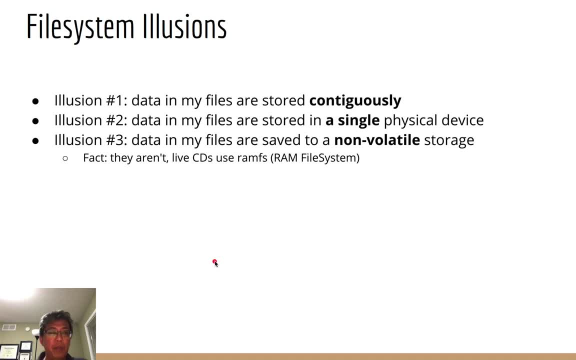 system to your computer. you may boot the operating system from a CD and at that point the operating system will not alter the current operating system on your hard drive. and in order for that installation process to work, the operating system may create a temporary file system on memory. 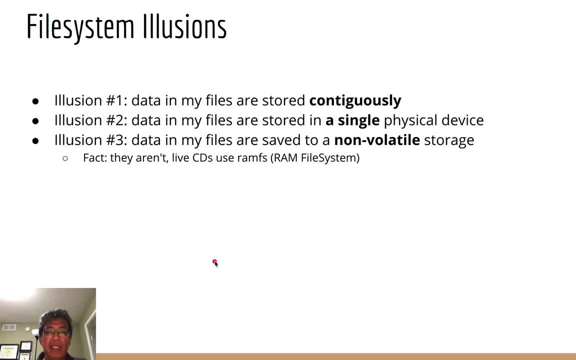 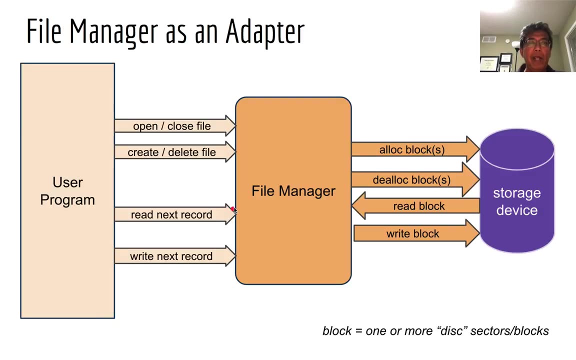 so in Linux, for instance, there is a type of file system known as RAM FS, because that file system is not persisted into your hard drive, but the file system exists only on your physical memory. among the main jobs of a file system is to translate system calls issued by your process to. 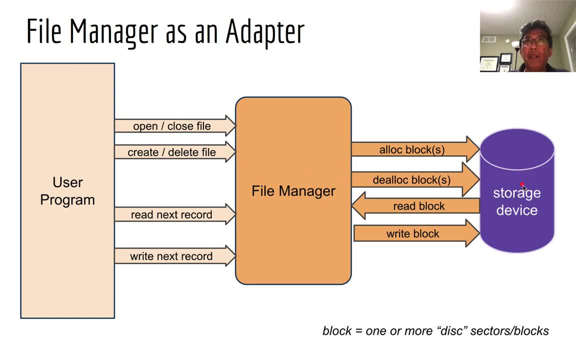 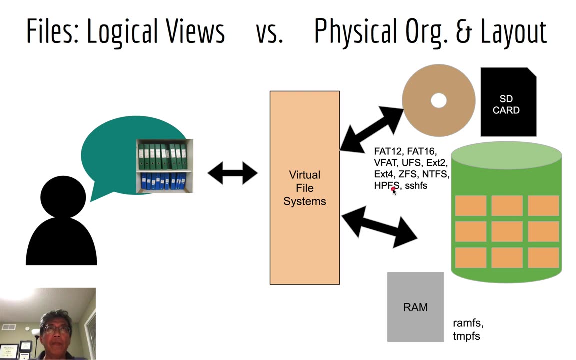 operate on a file or directory to lower level disk block operations. and again we're going to use the word disc when the underlying storage can be either a hard drive or a solid state drive. the programming model presented to the user allows the user to think that their files are documents organized nicely into different shelves, each. 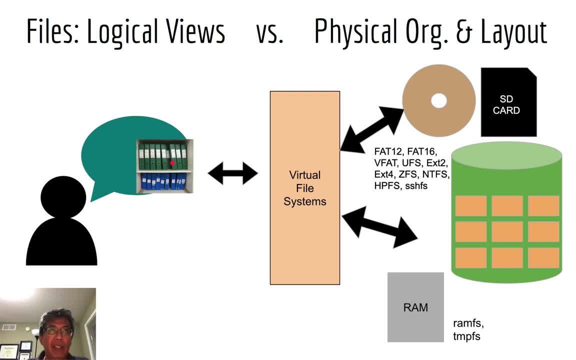 document is carefully labeled with the date when it is created, the document name and the owner, and so on. this programming model should work the same regardless of the implementation details of the file system. for instance, the actual file system may be either a vfat running on windows or a next exit 2 running on linux, and maybe the actual destination. 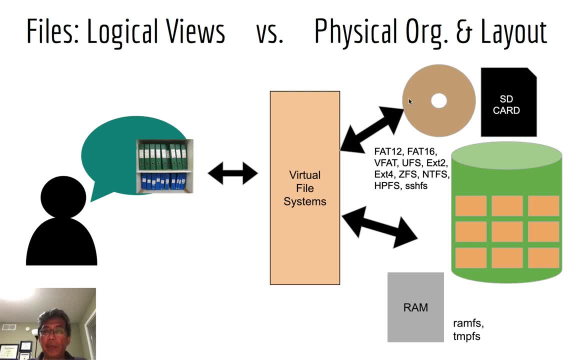 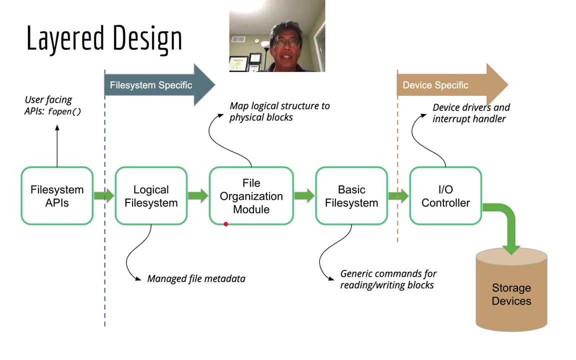 of the file is either a dvd drive or usb drive or a hard drive and many other details which are hidden from the user. when mainframe computers were widely used in the 60s, the most common storage devices were probably magnetic tapes and hard drives, and they were. 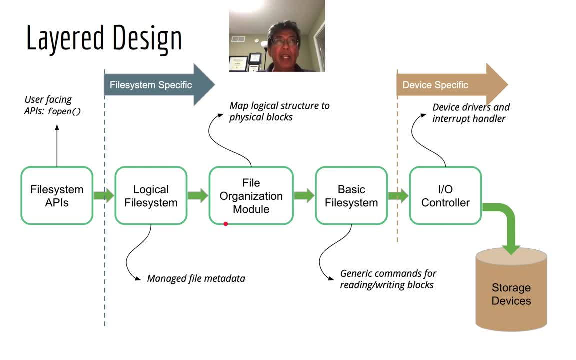 most likely manufactured by the same company. today the design landscape is more complex and operating systems must be designed to handle a larger variety of storage devices, like cd drives, dvd drives, flash drive, ssd, hard drives and also a variety of input output protocols to connect to these devices. like now you see usb version 1, version 2, version 3.. so this is why a layered 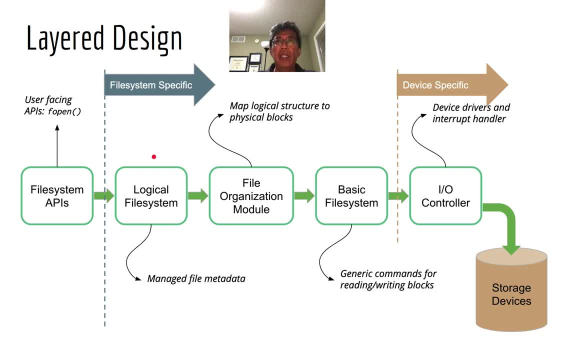 design is so complex. let's use an example of handling the f open system call from a c program. the syntax of f open should be the same regardless of the target operating system where the c program will run. so the first module in the layer design is the file system apis. 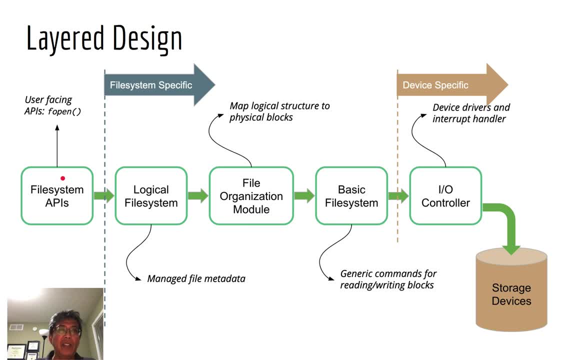 that present the same interface, regardless of the underlying operating system that imparts the c program. so let's use the idea of handling the f open system call from a c program implements the actual system call. the subsequent modules in the chain would be specific to each operating system variant. 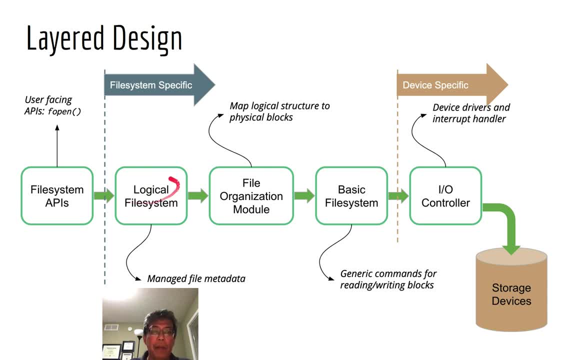 so, for instance, the first module inside the operating system file system deals with file metadata. for instance, at this level the os would verify if the requesting process is permitted to open the file, or the os will verify that the file can be opened in a particular mode because you can request a file to be opened. 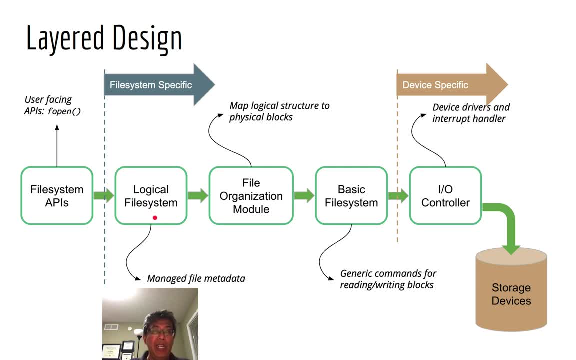 in binary mode, but the file is actually an ascii file or maybe the file is write protected and you try to open the file for writing. the next module deals with converting logical file pointer position to physical block number numbers. from the point of view- from the logical point of view- of the user, a file is associated with a file pointer. 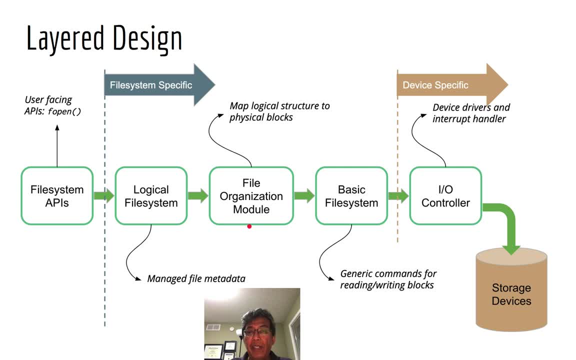 that can move forward and backward, but the physical implementation of moving the file pointer backward or forward will translate to which block will be read from your storage device. the next module, basic file system, is responsible for managing the block read- write operations and direct these operations to the right. 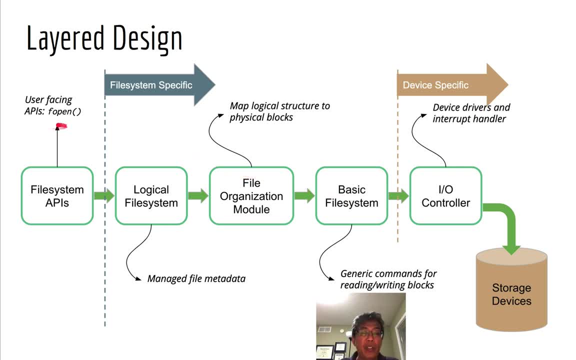 destination, because perhaps the file that you try to open is actually on a cd or maybe on a hard drive. that's why the basic file system is responsible for directing the basic block operations to the proper device. the last module, which is called the io controller, or sometimes we call it. device driver is specific to each device because, for instance, io commands for transferring data from a usb drive- flash drive- is maybe different from io commands from transferring data from a dvd drive in order to support all its internal operations within each module. in the later design, earlier the operating system works with a number of 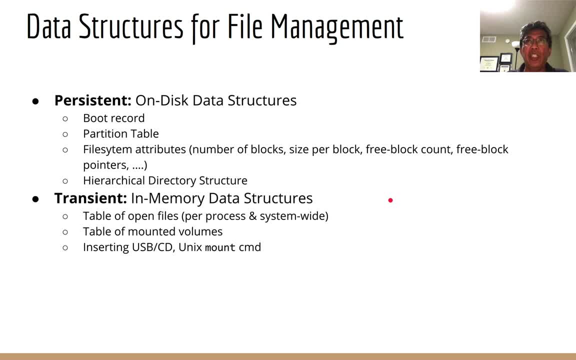 data structures. some of these data structures are to be persisted on the storage device, like the file metadata, the multi-level tree structure of the user directory. in addition, the operating system also maintains a few in-memory data structure that are not persisted to the storage device, for instance: 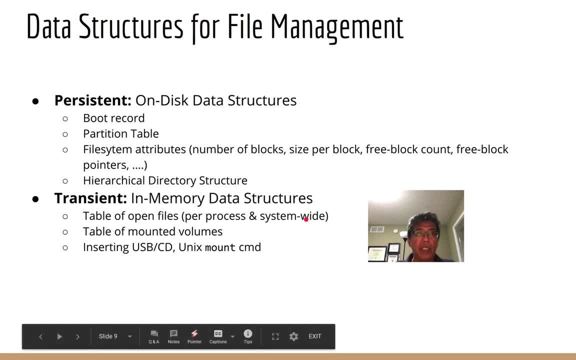 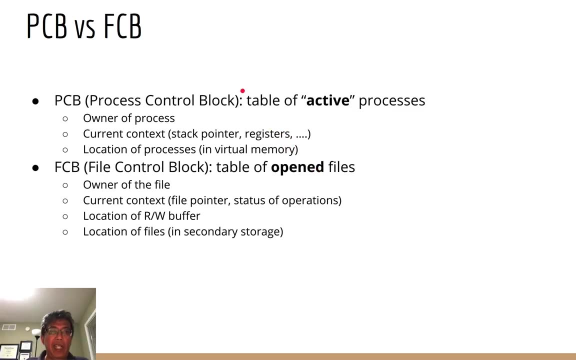 there will be tables to keep track which files are currently open by user programs or which user volumes are currently mounted when, let's say, you inserted your usb drive to your computer. these tables in the operating system are also known as control blocks, so for instance, for managing processes. 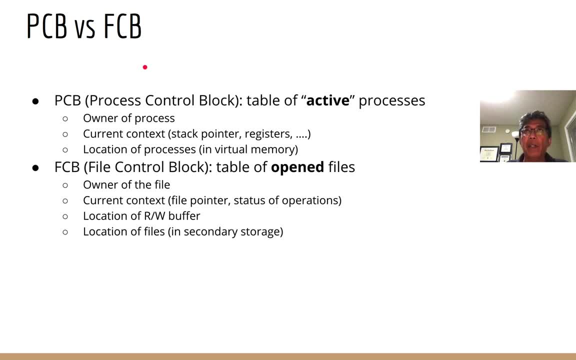 in your system. the operating system uses a table called process control block, which holds important information like process id, memory use, the amount of cpu, time, process priority and so on. same thing for managing files. the operating system will keep a table known as file control block. this table will hold important information such as: 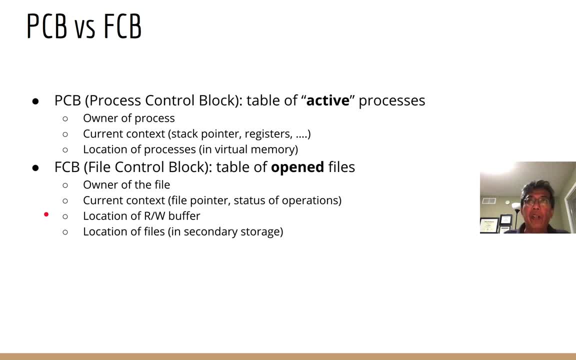 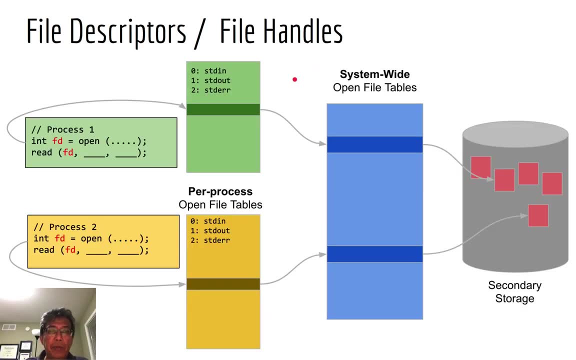 the file owner, file size, the buffer location, the current file pointer position and the data structure, and so on. just to emphasize the two types of table that may be maintained by the operating system, this page shows you two programs, process one and process two, in green and in yellow. 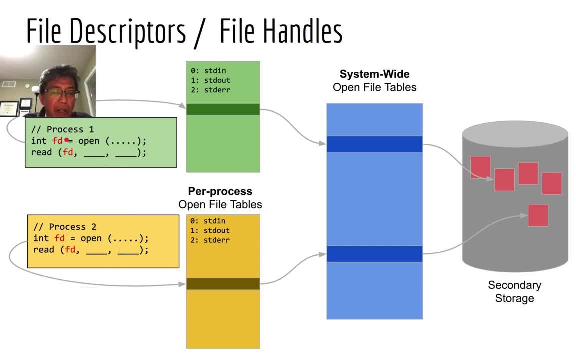 and let's say process. one uses the open system call to open a file and, if you remember, open is a function that return a file descriptor. and for the green process, the system will create a table. this is what we call per process: open file table. same thing for the yellow process. 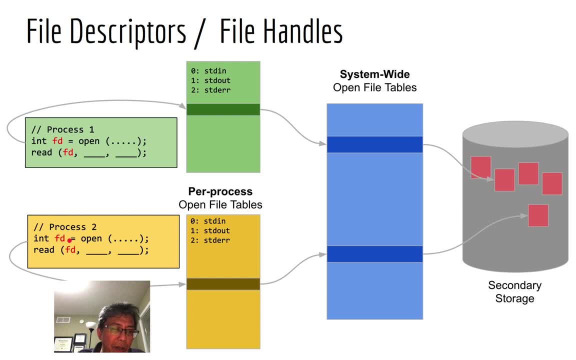 when the yellow process uses open to open a file, the system will create another table specific to that process. so for this example, you will see two tables, one per process. but in addition to per process open table, the operating system will also maintain a global table or a system-wide table to keep track. 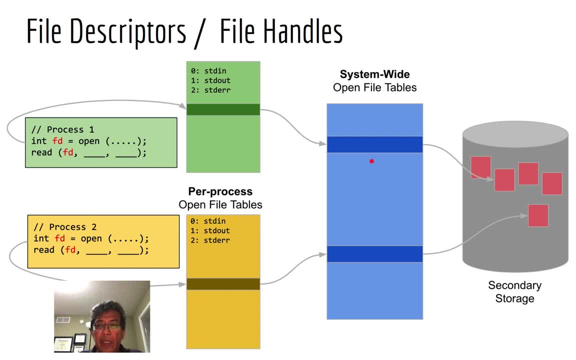 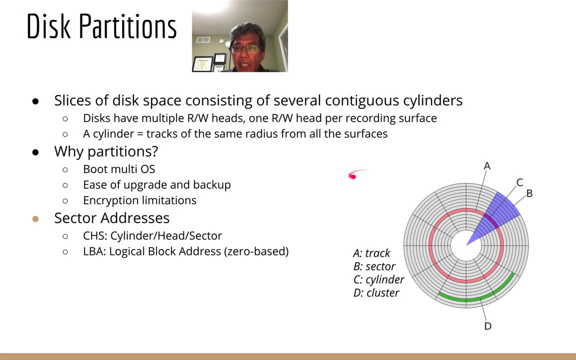 of all open files in the system. in the previous module we talk about disk partitions, but let's look at the details of different terms used in a hard drive. so in a hard drive data are recorded into concentric tracks, so the red circle here is a track. 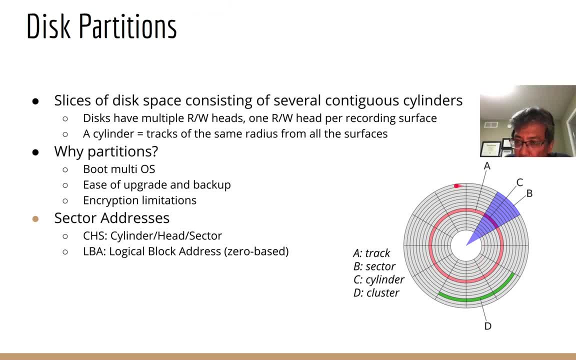 so usually track zero begins at the outer circle of your disk and track one is the next one, and so on. a track is usually divided into several sectors, so in our example we see 12 sectors per track. in a typical hard drive you will see several disks stacked into one main spindle. 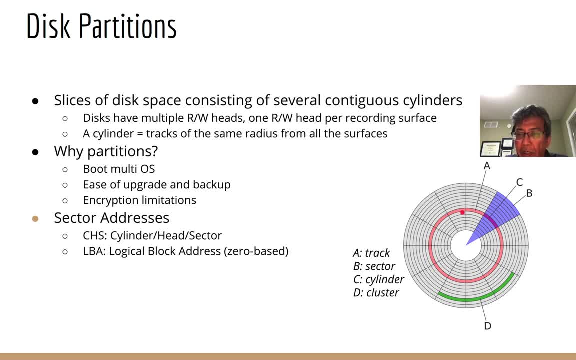 so if you take one track from the first plate and the same track number from the second plate and so on and so forth, you will get a cylinder. so a cylinder is practically a collection of track from different plates. now it's also common to see several adjacent sectors. 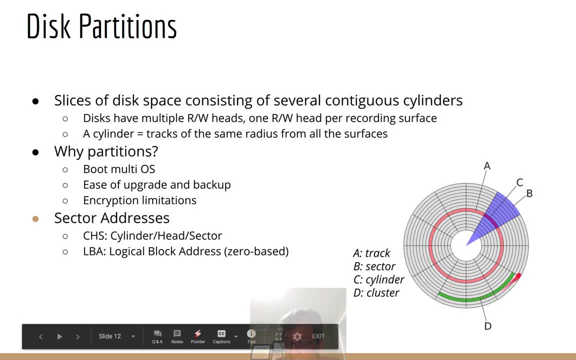 are combined into one cluster. so why do we create a cluster in a hard drive? Why do we create multiple partitions in a single hard drive? well, the most common reason is for us to install multiple operating systems on the same hard drive. so probably you want to answer both Windows and Linux at the same time. 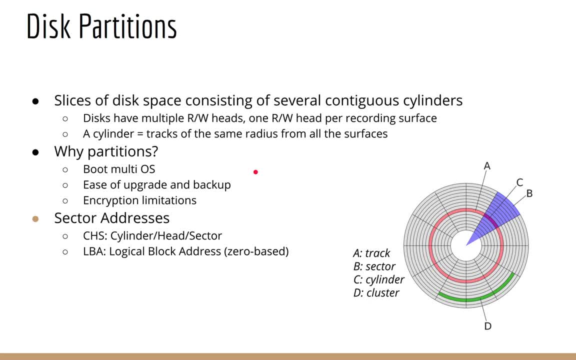 and also by dividing your hard drive into partitions, you can create backup of different partition at different time. so, instead of making backup of the entire disk, you can use the system as a data container which you can use to create backup of different partitions at different times. so, instead of making backup of the entire disk, you can use it to create backup of multiple systems. and whether you use the system or not, 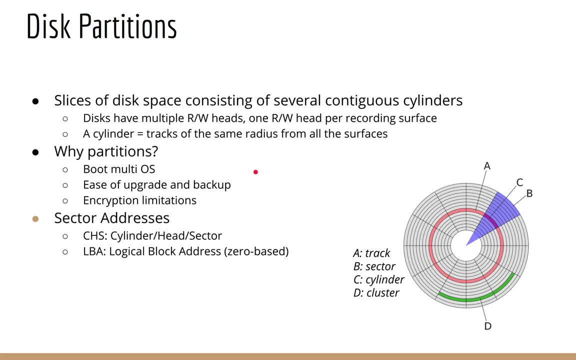 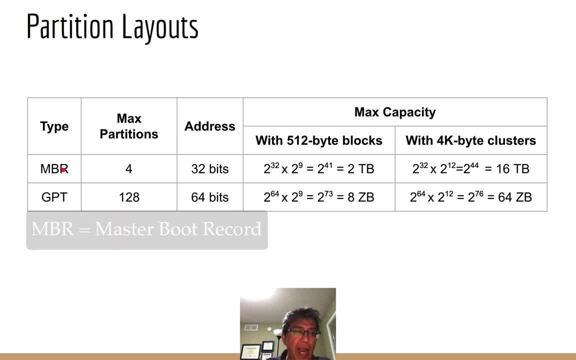 can just create a backup of a particular partition. So the two types of partitions commonly used today are MBR Master Boot Record and GPT GUID Partition Table. MBR is the older spec that allows only up to four partitions and it uses 30-bit address. 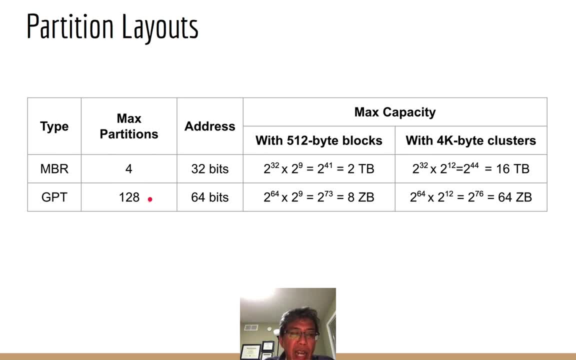 The newer spec GPT allows you to create as many as 128 partitions and it uses 64-bit address. So using this number, you can estimate the total capacity of your hard disk. So let's assume that your hard drive is formatted. 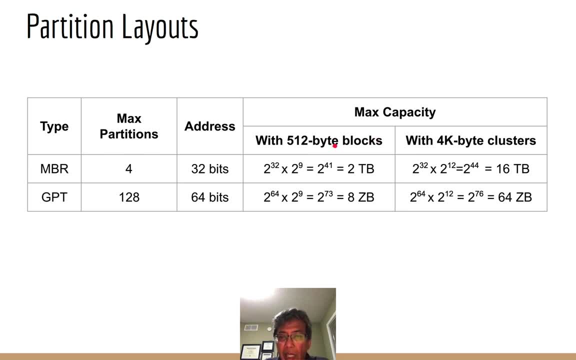 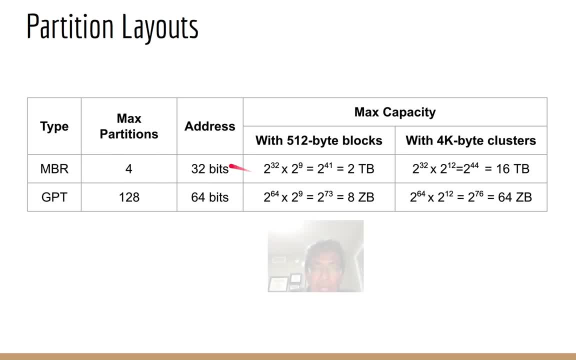 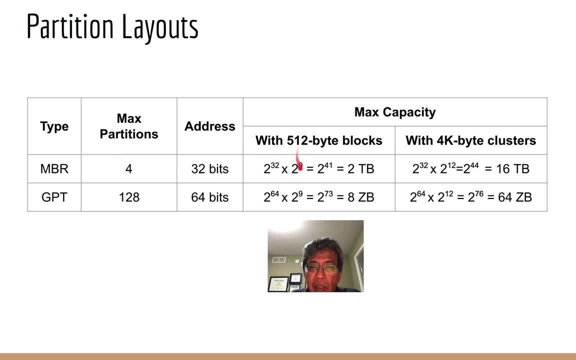 And each block is 512 bytes, or two to the power of nine. If you multiply the two numbers together, you will get two to the power of 41, which is equal to two terabytes. Now, with the GPT, because it's. 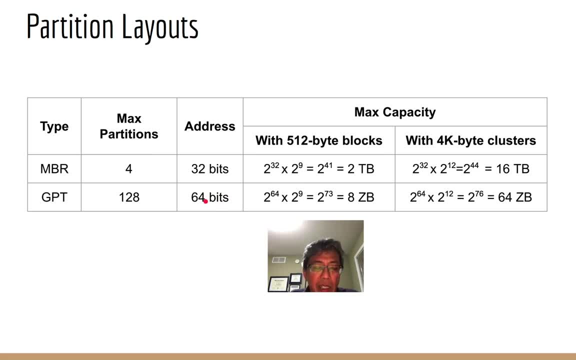 gives you 64-bit address. that means the hard drive can have as many as 2 to the power of 64 blocks. And again, if we are using 5 12-byte blocks, then the total size would be 2 to the. 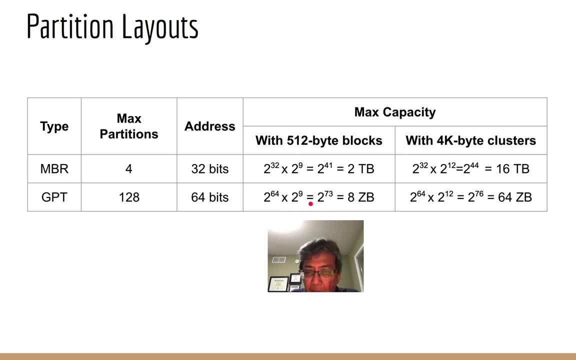 power of 64 times 2 to the power of 9, that will give you 2 to the power of 73, and that number is equal to 8 zettabytes, which is a lot. What if the hard drive combines adjacent blocks into? 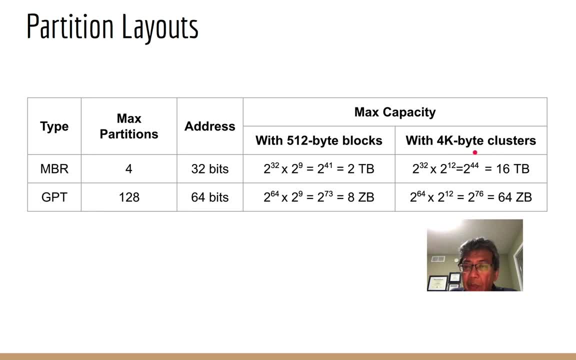 a bigger cluster. So instead of having individual blocks of 5- 12-bytes, what if the hard drive combined several blocks into a bigger size cluster of 4k bytes? And again using these numbers, then you can see the capacity. 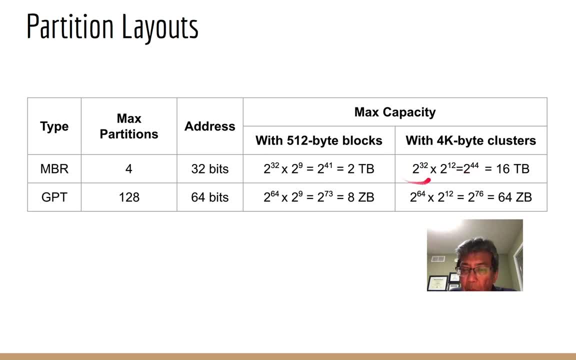 would be 2 to the power of 32.. How do we get this number? Because we are using 32-bit address, so that means the disk can have as many as 2 to the power of 32 blocks. but now the size of each. 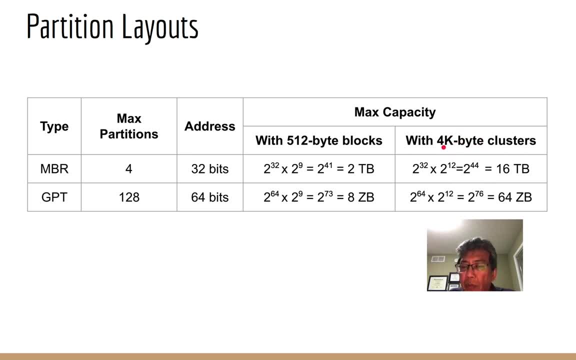 block, or, in this case, each cluster is 4k, and 4k is equal to 2 to the power of 12.. If you multiply the two numbers together, you'll get 2 to the power of 44,, which is equal to. 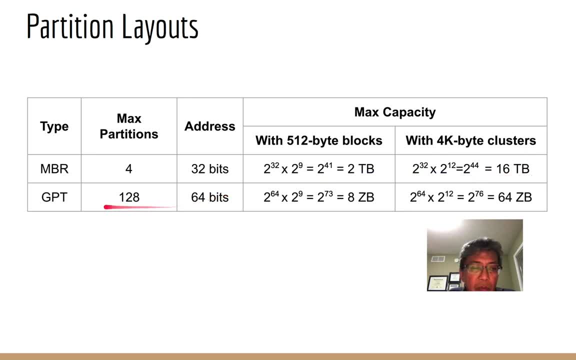 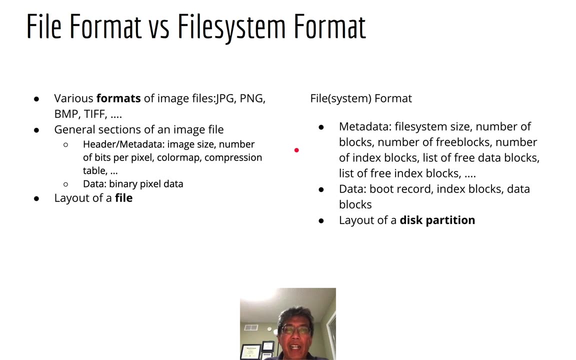 16 terabytes, And again for the GPT drive. you can do the math and it will give you 64 zettabytes. So why do we see so many different file systems like NTFS, EXT2,, EXT3, VFAT and so on and so forth? 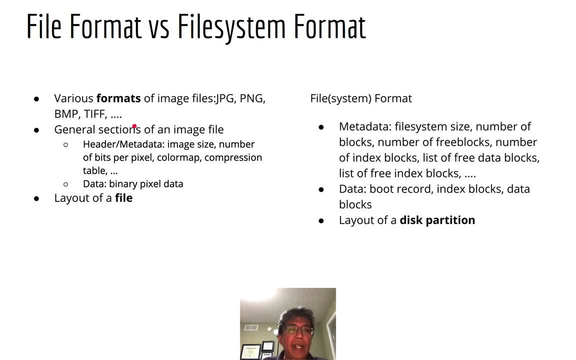 To understand this concept, let's first look at image formats. So we know different image formats, like JPEG and so on and so forth, but we don't know how much image format we can get out of this: png, bmp and so on. so in general, when you look at an image file, the important metadata in that file, 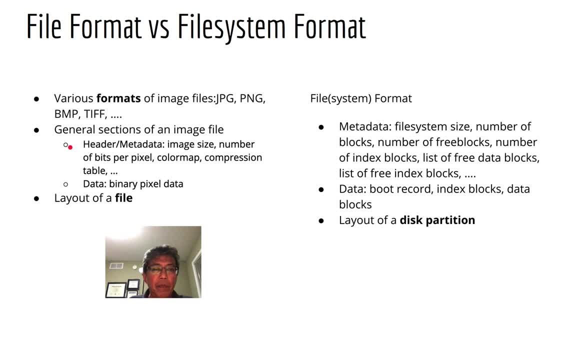 would be the image size, like how many columns, how many rows in the image, how many bits assigned per pixel, what is the color map, what is the compression table and, of course, the binary data of the image itself. if you read the spec of these image format, you will see. the spec will tell you how these data 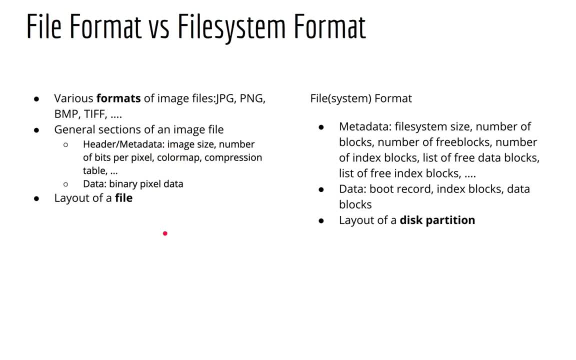 are laid out inside an image file. so, for instance, for a jpeg, maybe the height of the image is found in offset 10, maybe the width is offset 12, but for a png, maybe the width of the image is in offset 4, maybe the height is in offset 6.. so a file format basically specifies the layout of an image file. 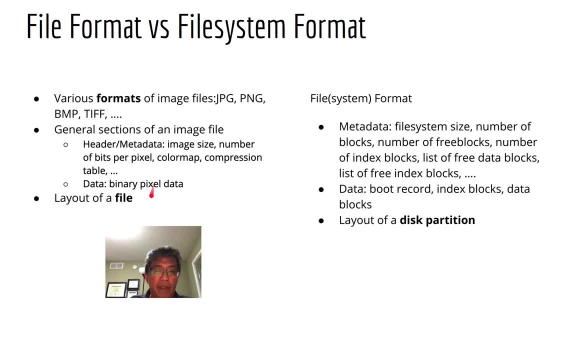 how different data is stored inside the file. so, using this analogy, a file system format is basically the same. so if you look at a file system, the important metadata for a file system is like the size, the total size of the file system, how many blocks allocated to the file system, how many free blocks, how many index blocks. 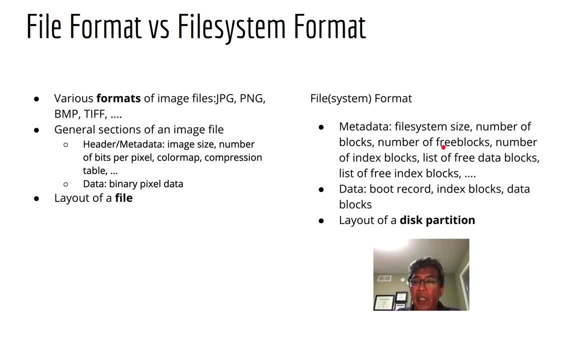 how many files are there, what is the structure of the directory, and so on and so forth. so then when you create a file system, basically you design the layout, how a disk will be organized into different parts. so if you compare the two again, the image format is like how to lay out. 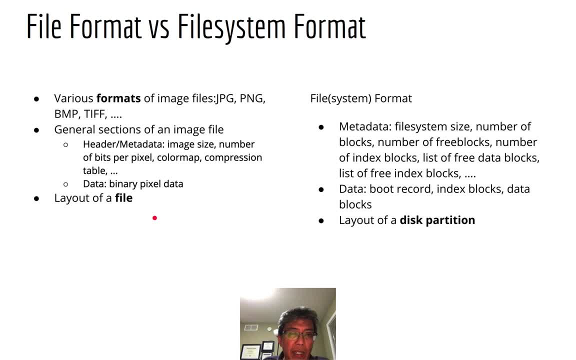